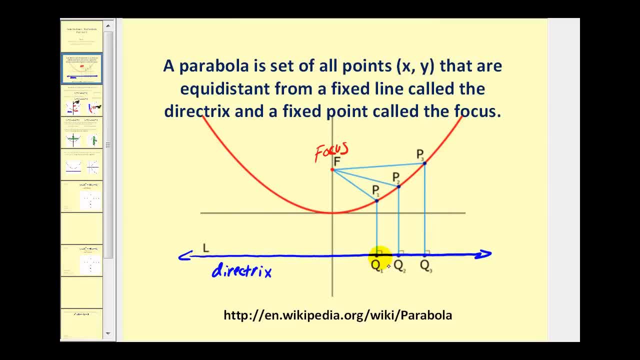 distance from the point as they are to this horizontal line. So the length of this segment here would equal the length of this segment here. The length of this segment here would equal the length of this segment here, And the same for this segment and this segment, And the same would be true for any point on this. 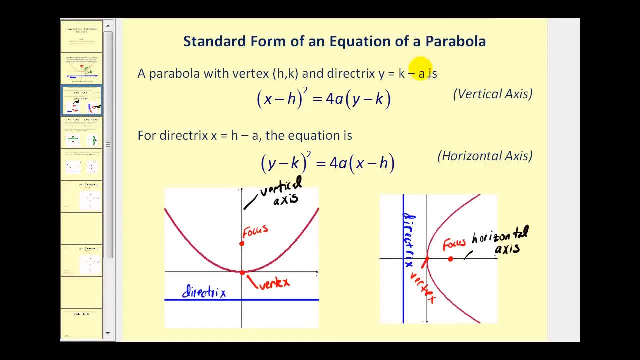 parabola. Before we take a look at the standard form of an equation of parabola, let's go and take a look at the graphs of parabolas. Some parabolas have a vertical axis, as we see here on the screen. 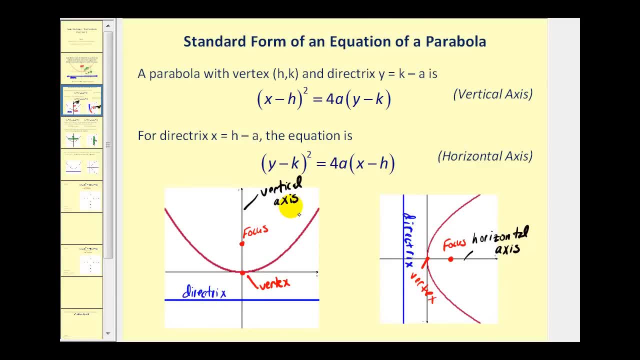 On the left- sometimes this is called the axis of symmetry- And on the right we have a horizontal axis or horizontal line of symmetry. Remember, this is the line where, if you were to fold the parabola across that, it would match up perfectly with the other half, Or we can say it's symmetrical across that line, As 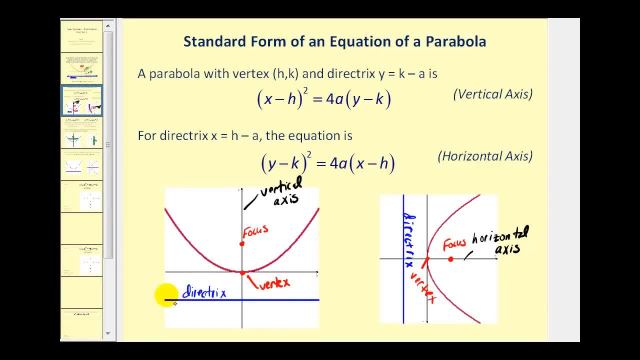 we saw in the previous screen, every parabola will have a directrix as well as a focus, And then, lastly, every parabola also has a vertex. It's the only point that is on the axis and on the parabola. Let's take a look at the. 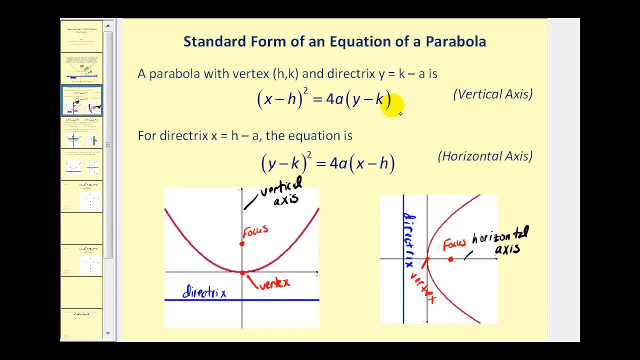 standard form of an equation of a parabola. now, If the parabola has a vertical axis, as we see here on the left, it will be in this form. Notice, the x part of the equation is being squared. So whenever the x part of the equation is, 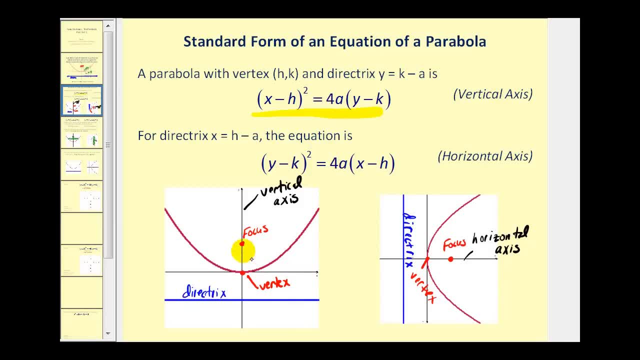 being squared, we will have a vertical axis, as we see here. This shouldn't be too hard to remember, because we have graphed parabolas in the form of y equals x squared before, And they always either open up or open down. The coordinates of the vertex of the parabola will be h- k, So 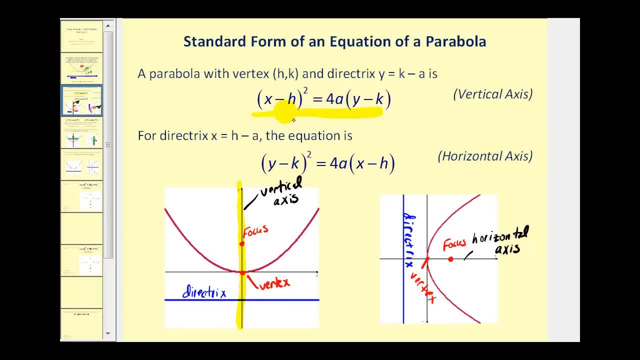 we can determine the vertex by inspecting the equation. Next, we should be able to look at the equation and determine the value of a, And that's going to be extremely important because a will tell us the distance from the vertex to the focus, And it will also tell us the distance from the vertex to 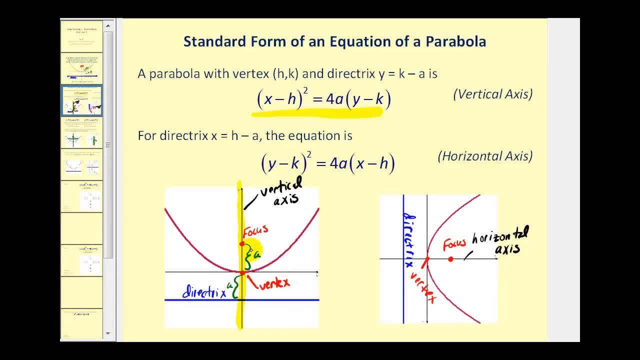 the directrix. So if this was a graph, we could determine the coordinates of the focus by adding a to the y-coordinate of the vertex, And we could find the equation of the directrix by subtracting a from the y-coordinate of the vertex. Now, if the y part of the 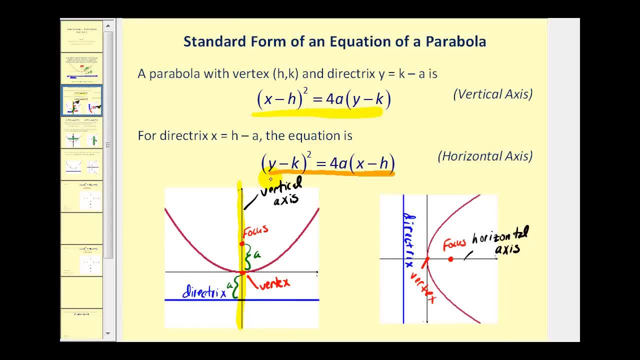 equation is being squared. This indicates that we will have a horizontal axis, as we see here on the right, But the vertex will still be h, k And a will still tell us the distance from the vertex to the y-coordinate of the vertex to the y-coordinate of the vertex. 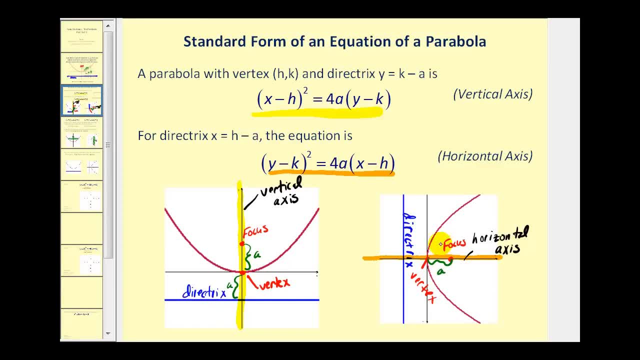 from the vertex to the focus, as well as the distance from the vertex to the directrix. But in this case, if this was our graph, we would add a to the x-coordinate of the vertex to find the focus and subtract a from the x-coordinate of the vertex. 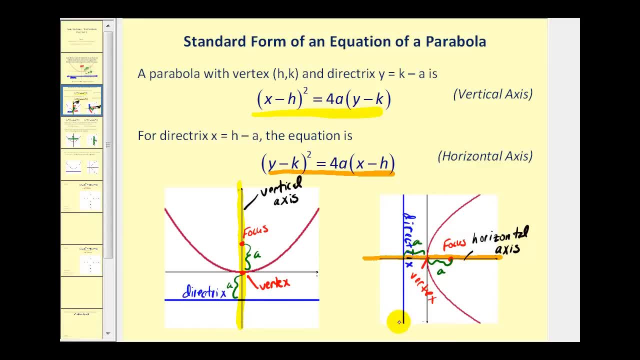 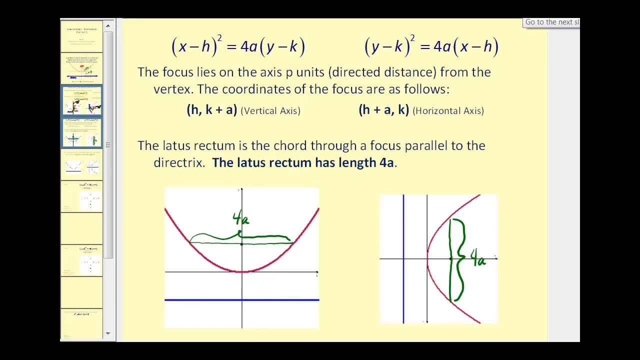 to determine the equation of the directrix. So, based upon whether we have a vertical or horizontal axis, that'll affect whether we add or subtract a to the x- or y-coordinate of the vertex. There's one more thing we want to mention before we try to graph some of our own. 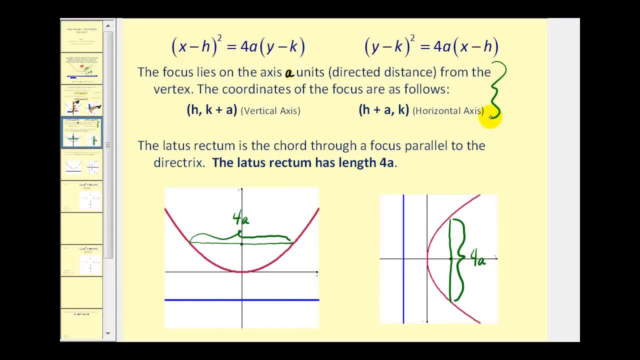 Now, these notes here just formalize what we just said about how to determine the coordinates of the focus, as well as the equation of the directrix. So the last thing we want to talk about is the lattice rectum, and this is the chord through a focus. 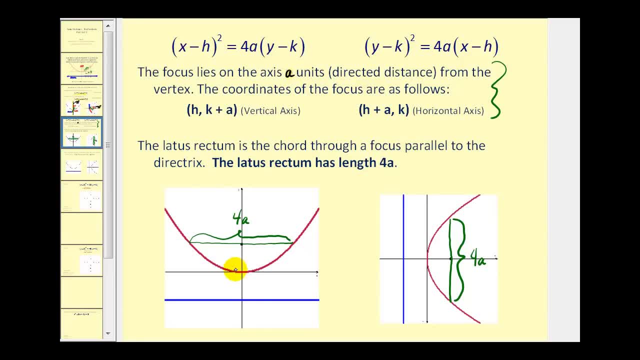 parallel to the directrix, as we see here in green, for a vertical axis and horizontal axis. And what's nice about that is it has a length of 4a and we can determine the value of 4a by looking at the equation in standard form. 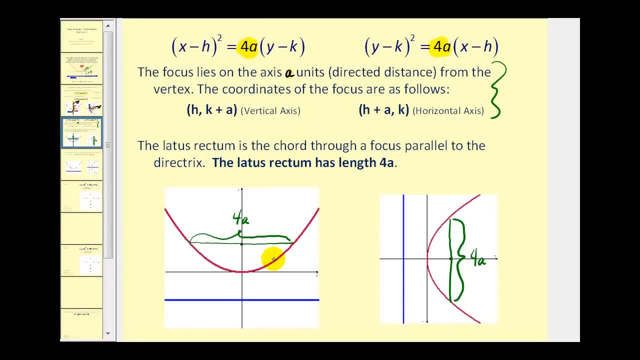 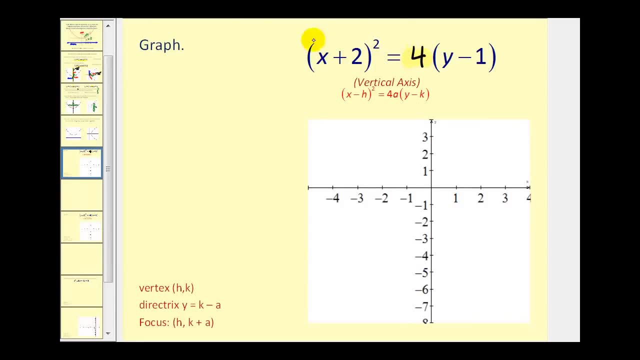 So this will tell us how wide or how narrow our parabola will be. Let's go ahead and take a look at a couple examples of our own. The first thing we should notice about this equation is the x part is being squared. therefore, we're going to have a vertical axis. 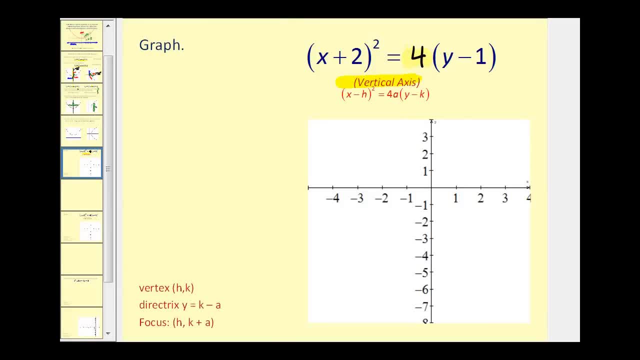 Next, we should be able to determine the coordinates of the vertex by looking at this equation. Remember, the vertex has the coordinates hk, x plus two. the x coordinate would be negative two, and if we see y minus one, the y coordinate would be positive one. 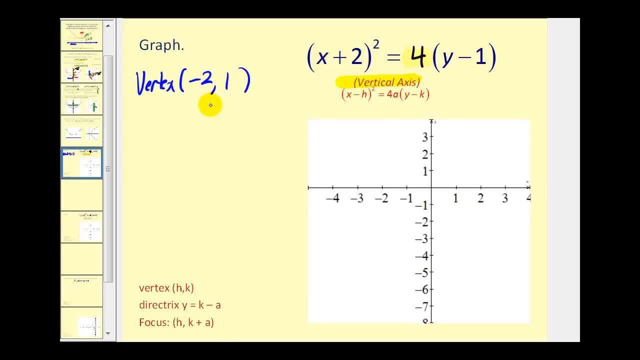 Next, if we can determine the value of a, we should be able to determine the coordinates of the focus as well as the equation of the directrix. Well, 4a is equal to four. therefore, a is equal to one. Let's go ahead and graph some of this now. 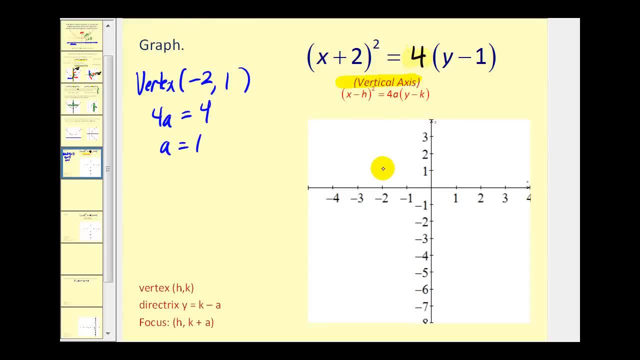 We're going to plot the vertex, the vertex at negative two one. Next, we know we have a vertical axis and it passes through the vertex. Let's go ahead and sketch that And this line would have the equation x equals negative two. 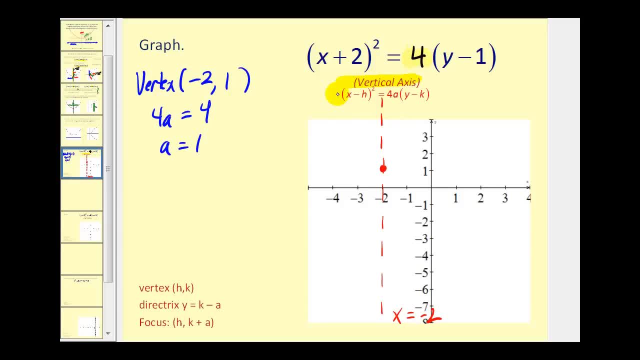 One thing we didn't mention before was if a is positive, this graph is going to open up. If a is negative, it's going to open down. So this graph is going to open up. Let's go ahead and write that down. 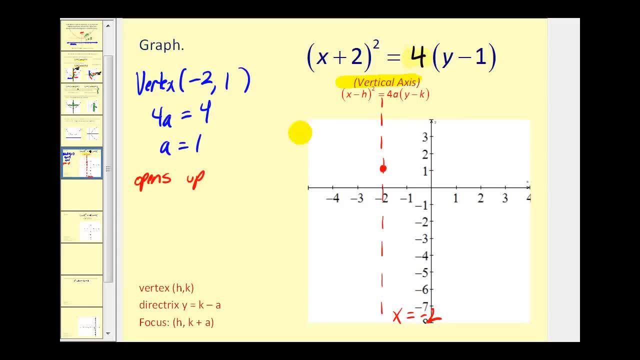 So if this parabola opens up, we know the focus will be inside the parabola and it will be one unit above the coordinates of the vertex. So we'll add one to the y coordinate to find the focus. So this would be the point. negative two, two. 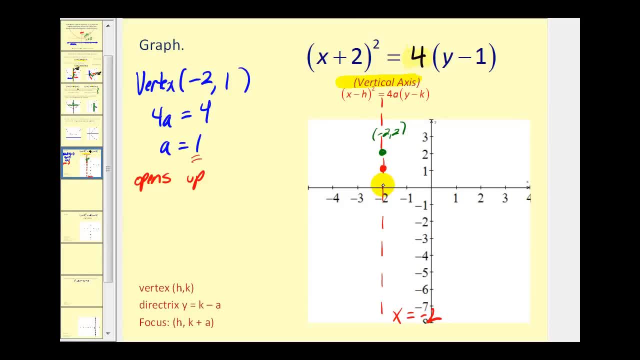 Now the directrix will be a horizontal line, one unit below the vertex in this case. So if we go one unit below the vertex, this point here would be one point on the directrix. so this equation here, so this line here would be the equation. 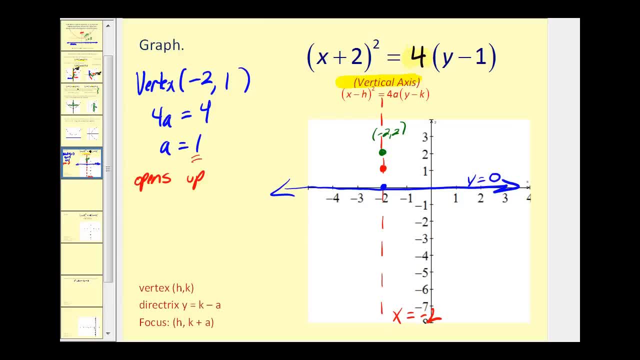 of the directrix and this would be: y equals zero. Now we know the parabola opens up, so it looks something like this, but we're not really sure how wide it will be. But now, if we sketch the end point to the lattice rectum, 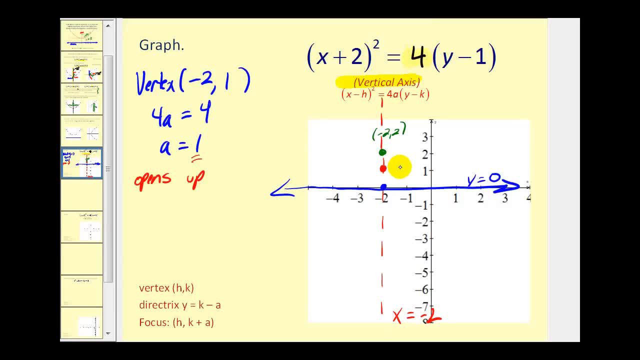 we'll have two more additional points on that parabola. The lattice rectum would have like one point below the vertex. so this is, two physical points have length 4a. so we're going to sketch a segment four units long through this green. 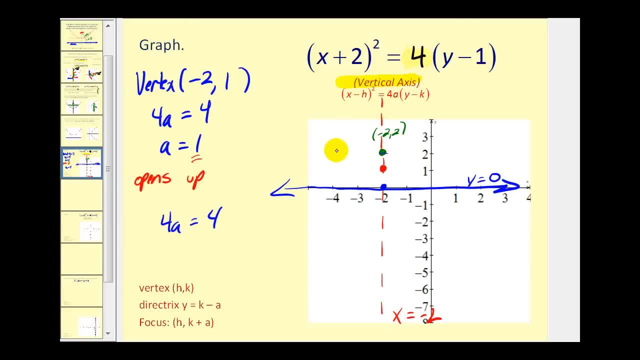 point parallel to the directrix, and that would look like this: So this end point and this end point are on that parabola, and that should be enough information to make a nice sketch. It would look something like this: Again, we have our directrix, we have our. 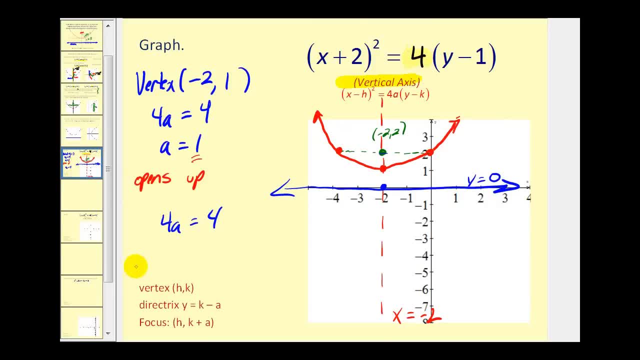 focus and we have our parabola Now. you notice I did include some notes down here, but I think if we can logically determine where the focus and directrix should be, it's going to be a lot easier than trying to memorize these notes based upon whether it has a vertical. 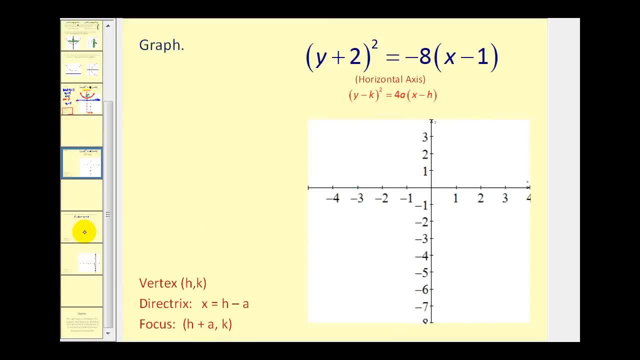 or horizontal axis. Let's go ahead and take a look at one more Notice. now the y part of the equation is being squared, which indicates we're going to have a horizontal axis. Our vertex will still have the coordinates hk, so the x coordinate will be positive 1, and the y coordinate will be. 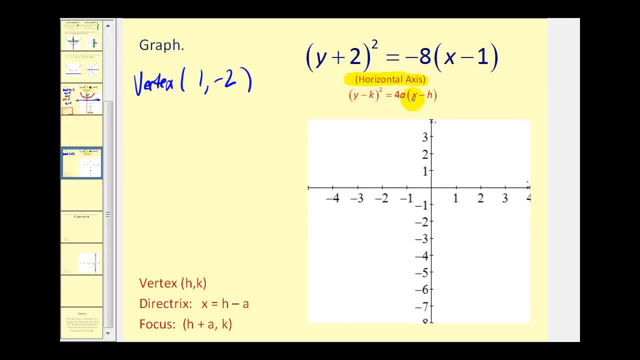 negative 2.. Let's go ahead and find the value of a. We know that 4a equals negative 8,, so that means a will equal negative 2.. Notice, now we have a negative value of a, and so what that means is that our parabola, instead of opening right in the positive direction, 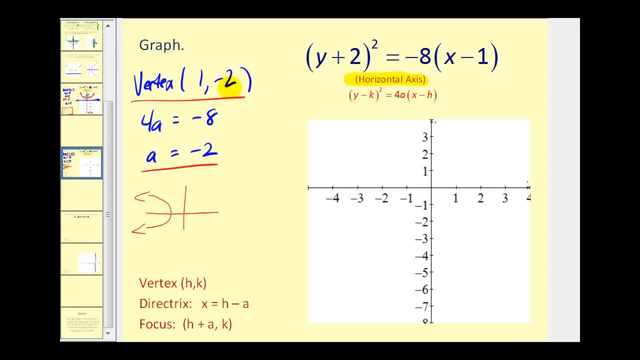 will open left in the negative direction. Let's go ahead and plot our vertex 1, negative 2.. Now we're going to take the absolute value of a now to determine the distance from the vertex to the focus. So the focus will be two units from the vertex and it will be 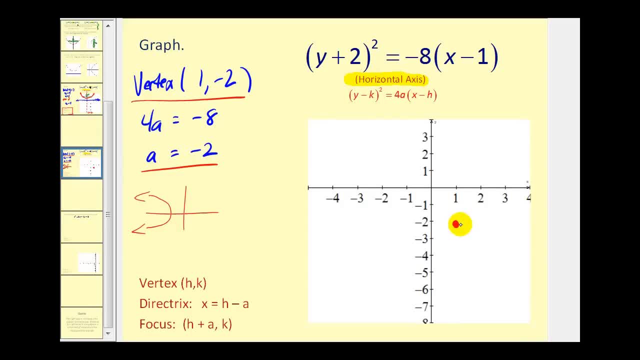 to the left because the parabola opens to the left. So we'll move two units to the left. This will be our focus: Negative 1,, negative 2.. And the directrix will be two units to the right of the vertex. 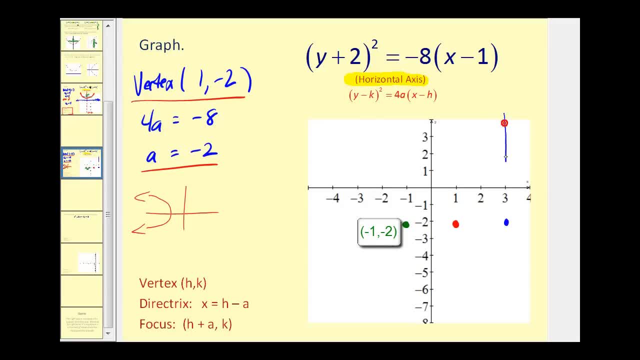 So it will pass through this point and it will be a vertical line And this is the equation: x equals 3.. And this is our directrix. So right now we only have one point on this parabola that we know opens to the left. But if we can sketch the lattice, rectum. 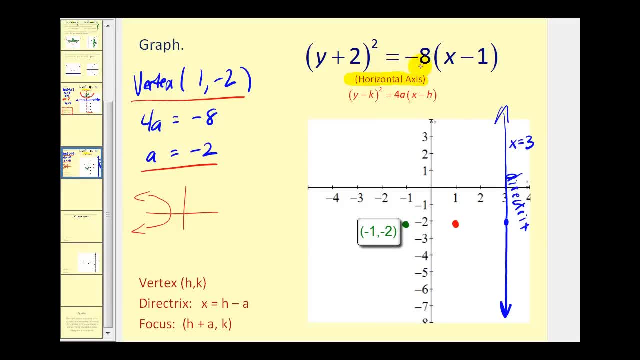 we can determine how wide or how narrow this parabola will be. The lattice rectum will have a length of eight units, So we're going to sketch a segment- that starts four units above the focus and stops four units below the focus. 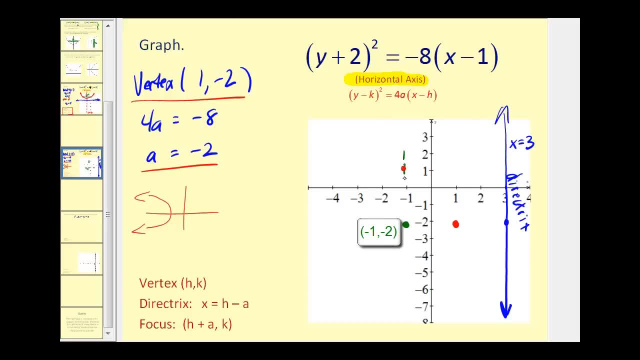 So it would look like this, And the endpoints of this segment would be two points on the parabola, As we see here. So our parabola will pass through these three points. It'll look something like this And something like this: